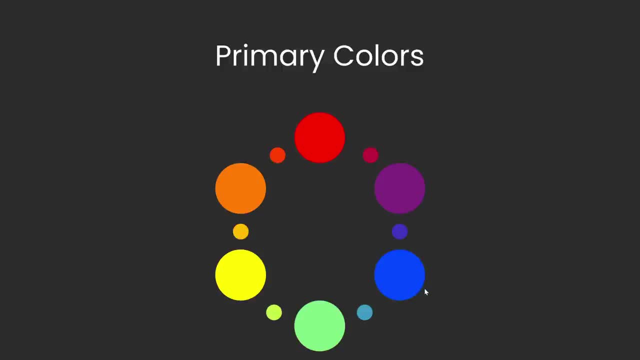 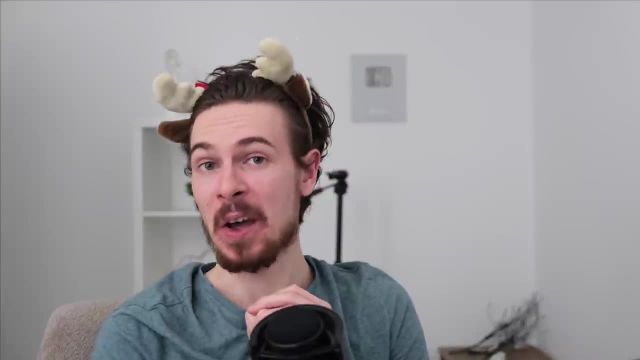 different shades of color are a type of hue, So the color of the color. Wow. Next up we have saturation. Saturation basically describes the intensity of a color. A very saturated color is going to look bright and alive, whereas a unsaturated color is going. 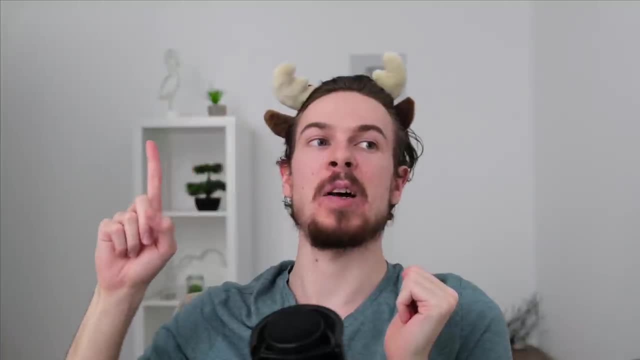 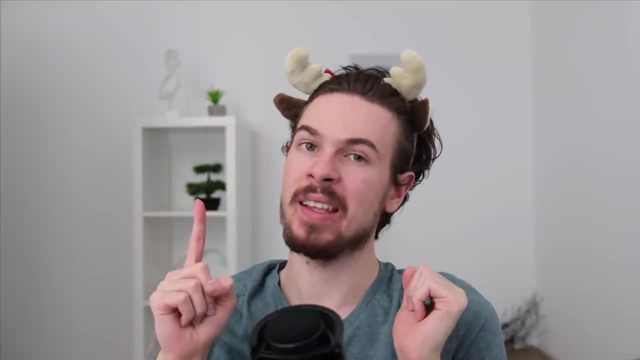 to look dull and boring. So, for example, this plant up here is very saturated, It looks bright, It looks very pretty, Whereas this plant right here it's still green, but it's just not saturated at all, And you can see this visually as well If you go outside, maybe. 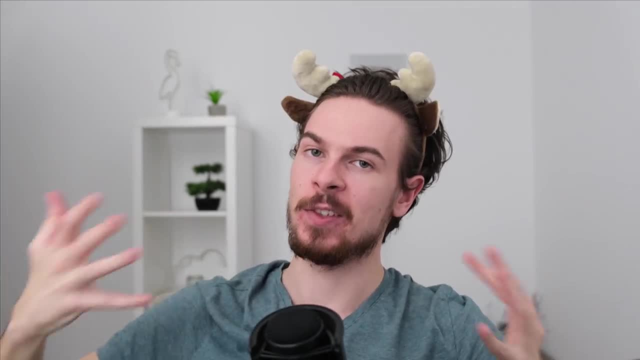 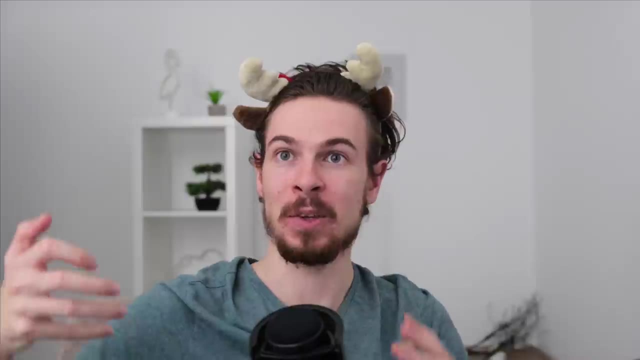 What I want to show you is that you can see that this plant up here is very saturated. What I want to say is: even brightness affects this. So if you walk outside at night and you look at the tree, you're not going to see that much green, Whereas if you go out and it's a bright. 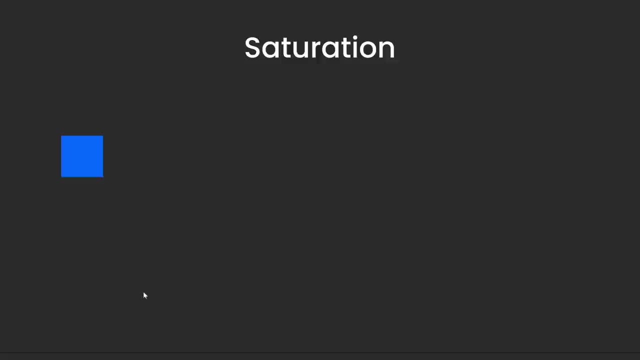 sunny day it's going to look green as f**k. So take a look. We picked a blue color here, And if I just basically drag down my slider all the way to gray, we desaturate this blue, And this is called a tone. All right, So take a look. 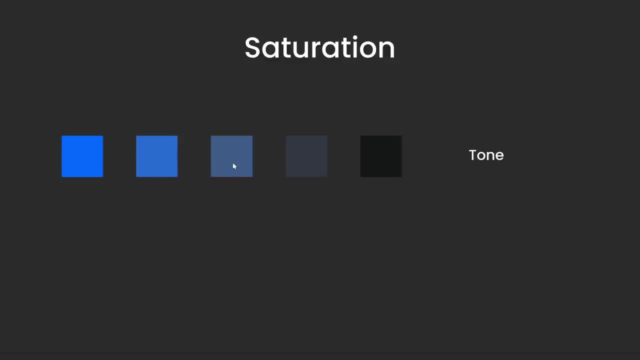 This is super intense blue. As we go lower it becomes duller and duller. Eventually we just get to a gray, All right, So completely desaturated. We cannot even tell that this is blue And, as I told you, lightness also affects our color. So if I add a bunch of white to it, or a 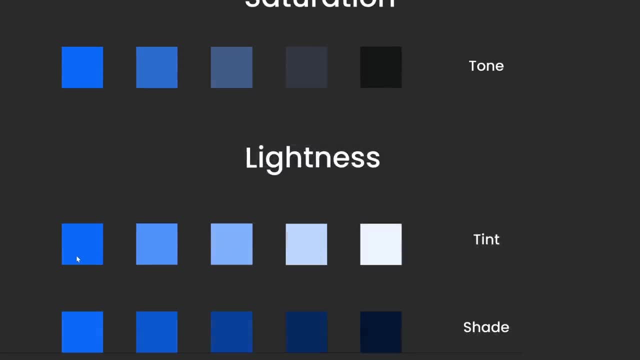 bunch of black to it, it's going to change as well. So take a look, here We add a bunch of white to it. It just opens up, gives us a different shade of blue all the way till we get to white, And here, with the shade, we just add a bunch of white to it. So if I add a bunch of white to it, 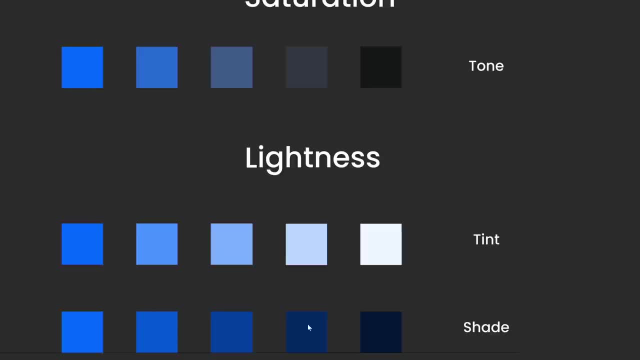 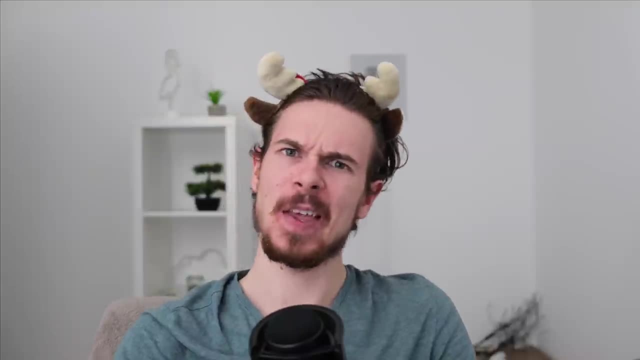 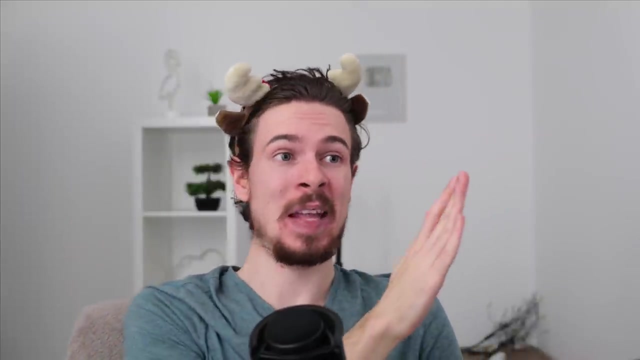 a bunch of black. So here we just go darker and darker and darker. If you think about it, we actually use these things before: Hue, saturation, lightness, HSL, That's what that means. So basically, H stands for hue, which goes from zero to 360.. So if we use that slider, 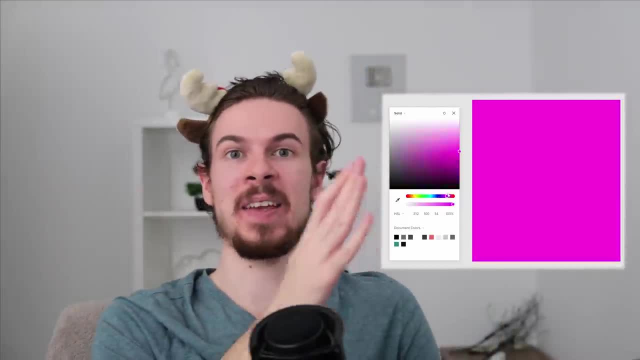 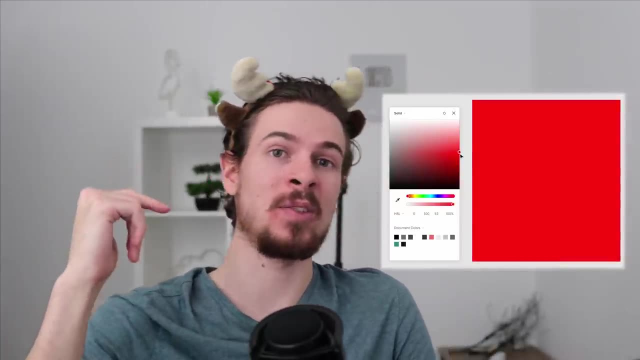 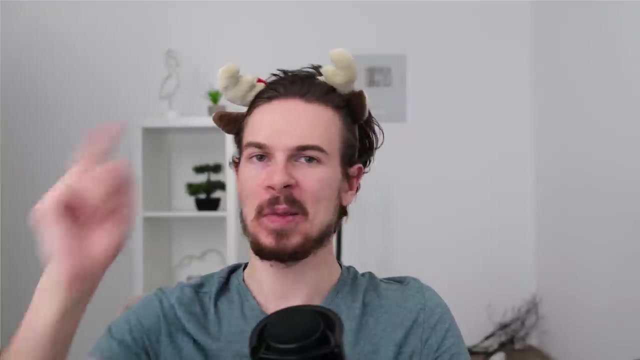 and go all the way to the end. we start from red and end up through the whole range all the way back to red. Then we have saturation, which goes from zero all the way to 100. And finally we have lightness, which basically goes from dark all the way to white. Next up: 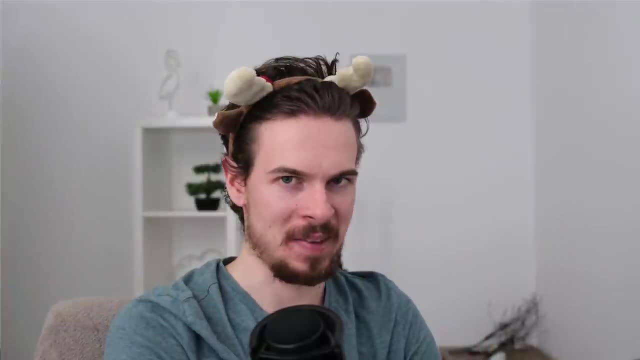 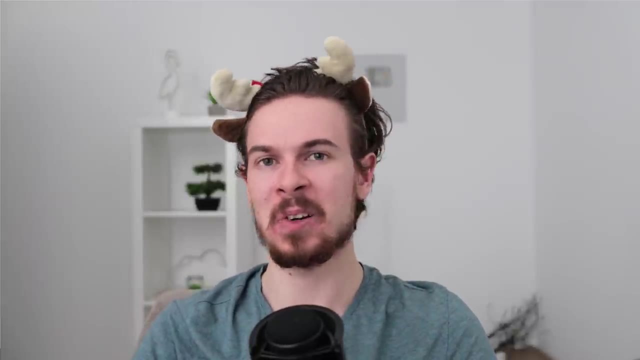 let's talk about color psychology and what each color means. So, when you're starting off with the design, which color are you going to pick? Well, it really depends. Let's start off with the color red. Color red represents passion, It represents love, It represents fucking and sex. 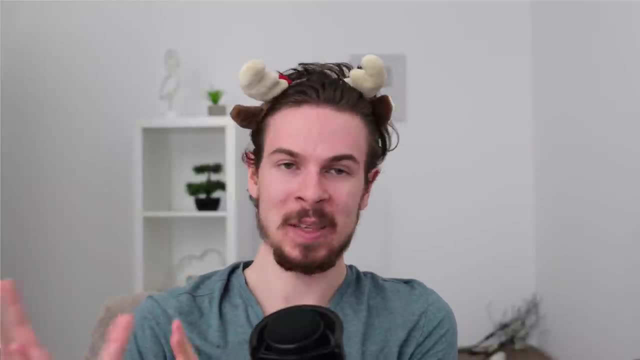 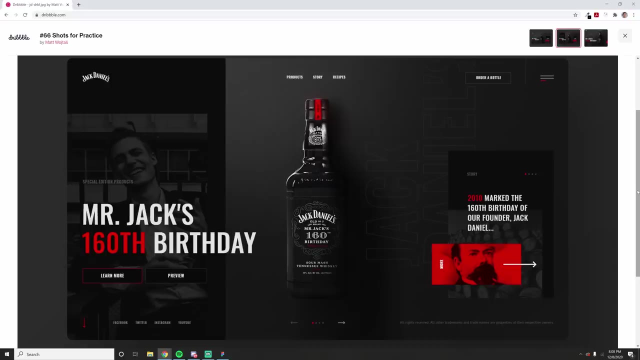 and all the I'm joking. Those are probably the positive things about it. right, Like very passionate, It can be Very exciting, energetic. So, for example, in this Jack Daniels design here, it uses a heavy, very saturated red color to give energy to this design and it's very attention-grabbing. 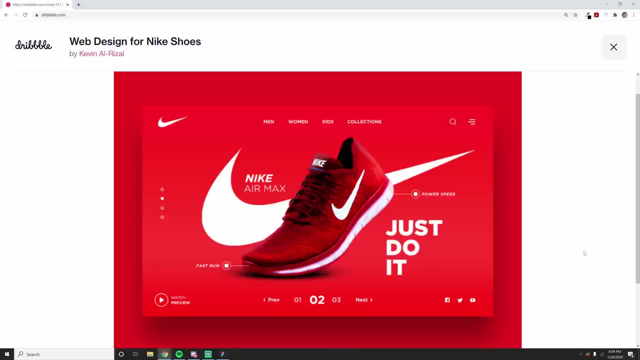 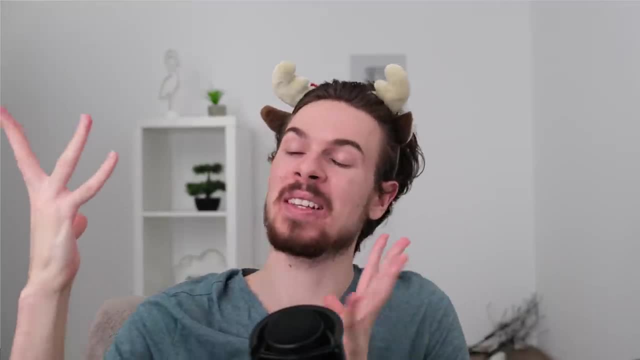 Again, you're going to see this in a bunch of sport designs, because that just says intensity and energy and passion about a specific sport. Next up, we have the color blue, which represents intelligence. It represents trust, security, intelligence. You're going to 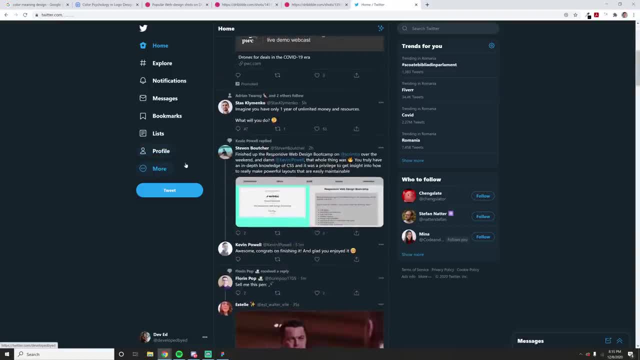 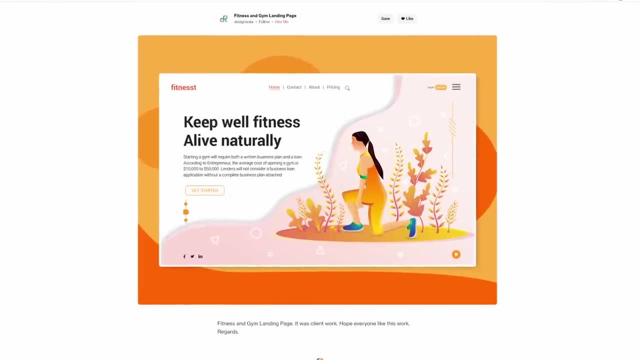 color the inside, so you're kind of going to color the inside the inside. This is what many of the other color technology tech websites use, especially Twitter and Facebook, So it's also the color of communication. The color orange gives you a very friendly vibe of happiness. 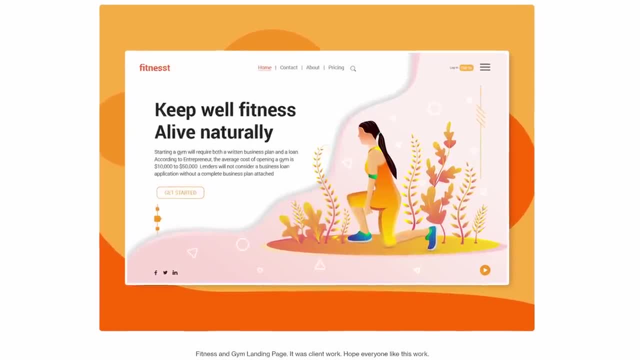 and joy. Imagine like there's a sunset going down and it makes you feel super warm inside. It gives you a sense of success and confidence. So this fitness website here is perfect with this orange color. The color green is probably one of the simplest ones to explain. 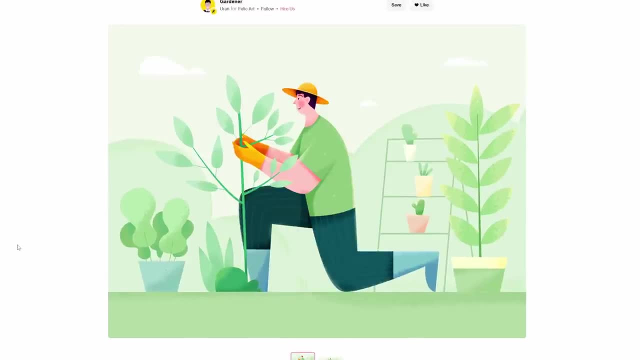 It's the color of nature. Some of the colors need to be color to them, So it might be technically modern. when you go to theipercom nature, so you're going to see this used a ton in websites or apps that are about health or about. 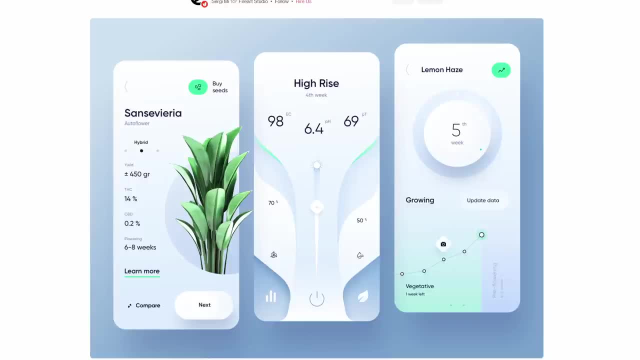 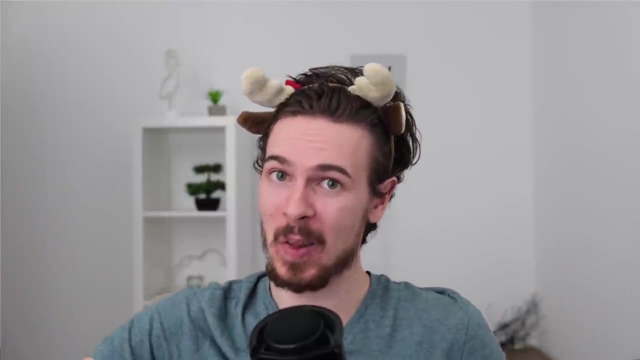 eating healthy diet apps, stuff like that. it represents peacefulness. it represents growth and money. so when you see that button and it's green, well it's. they want you to buy that. i also want to include non-color. so what is a non-color? it's the lack of a color, so white and black and 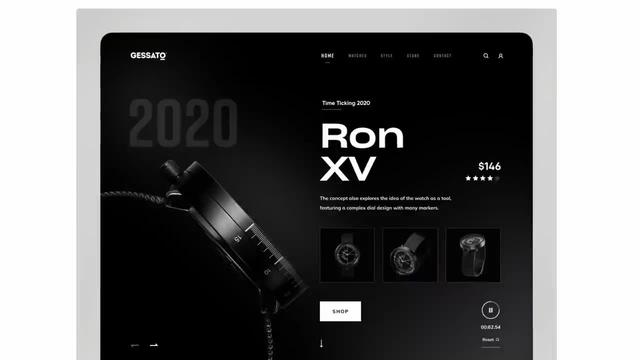 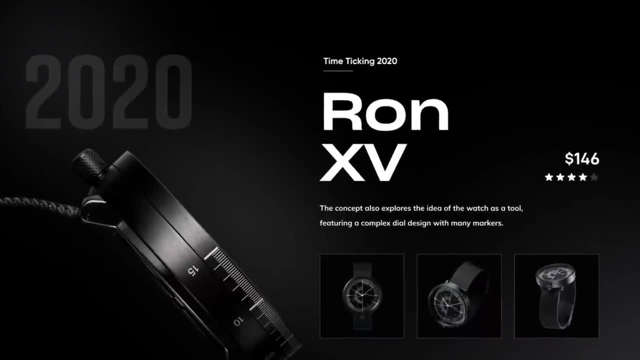 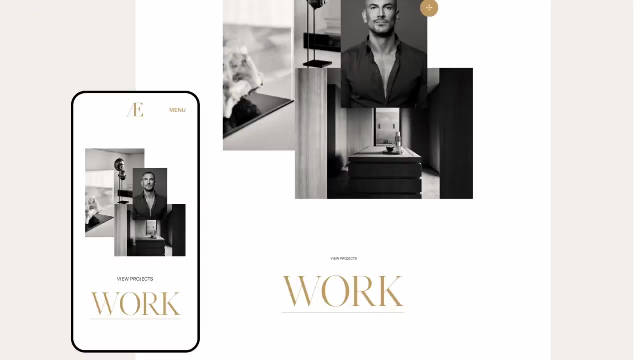 these also represent something so. black represents classiness and power often is associated with luxury, so you can imagine brands like nike and apple. they have black logos right, so they're very expensive. they often give off a feel of sophistication. white, on the other hand, can be very innocent. it can be pure, safe and clean. so just going black and white can often lead you to. 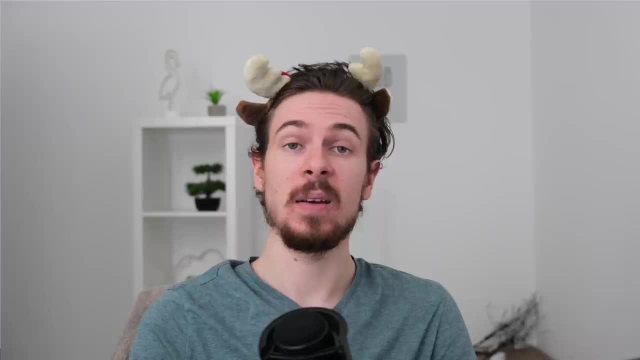 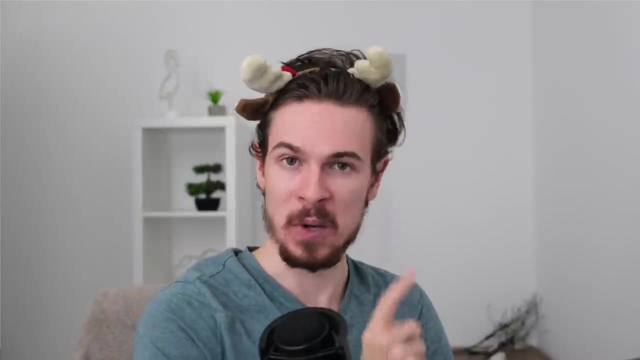 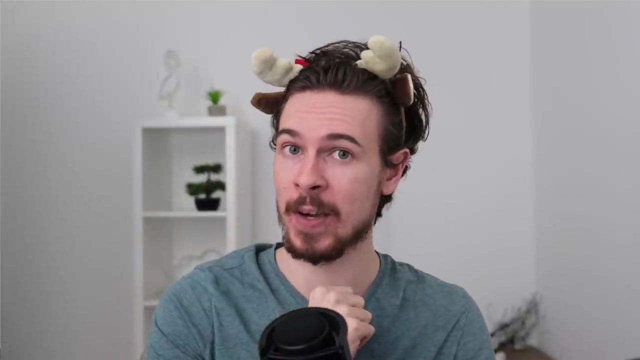 a very clean and sophisticated looking website. hey, so we learned what color to pick for our design. what if i want to use multiple colors? you don't need to use multiple colors. sometimes it's perfectly fine to use only one. you just take one color. let's say we're building a 420 website. 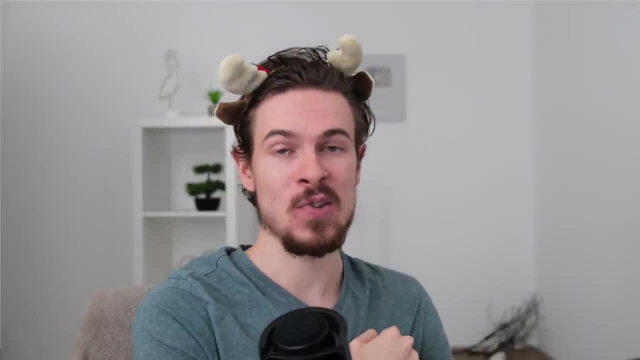 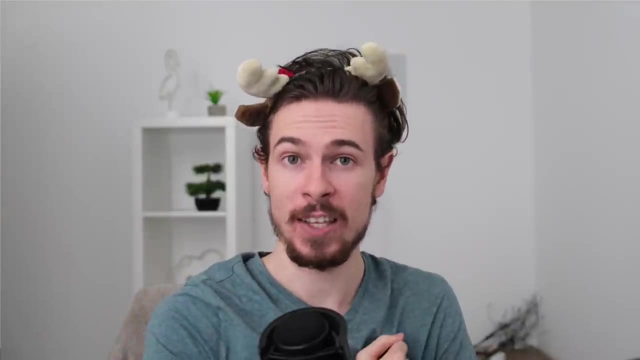 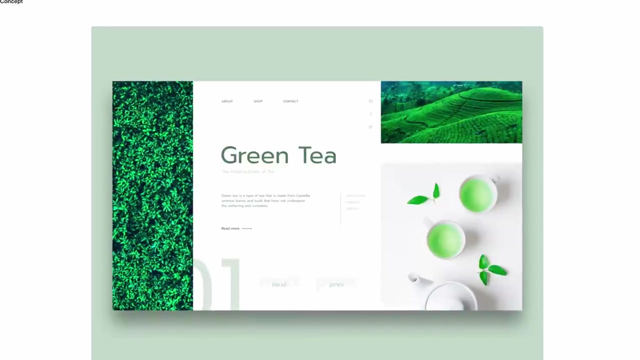 so we're going to be using the color green. now what i can do is just vary that color with saturation and lightness to achieve different kinds of shades of green, and this is what's called a monochromatic design. okay, so if we take a look at this one, we have green tea, for example. 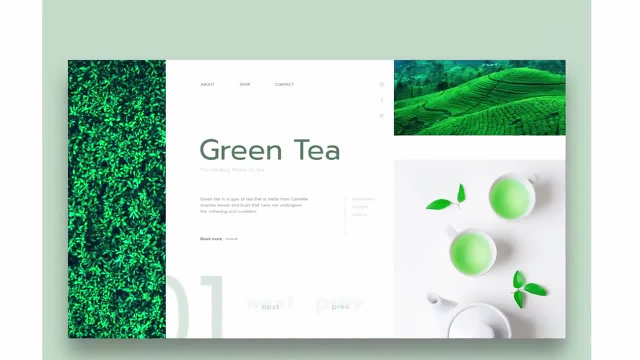 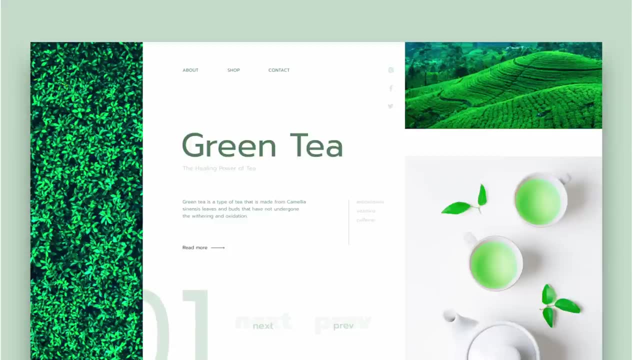 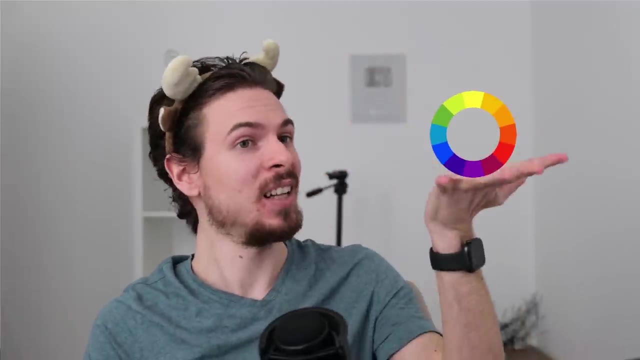 yeah, tea, and, as you can see, we have the header there. that's extremely dark, but it's still green. and then for the paragraph and the text there, we just picked a lighter shaded green and it still looks fantastic. okay, you still want to use a different color? then just grab the color wheel and spin it. 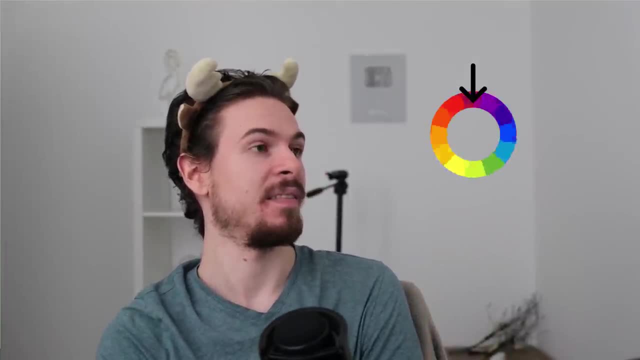 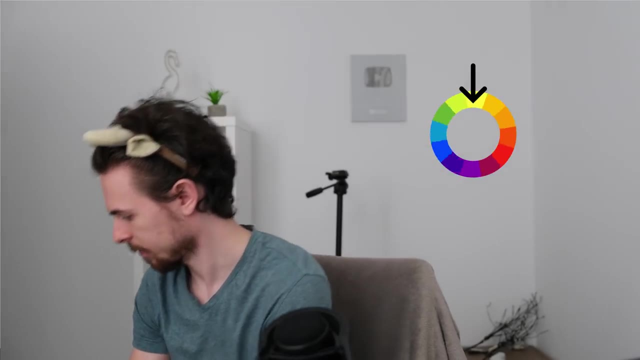 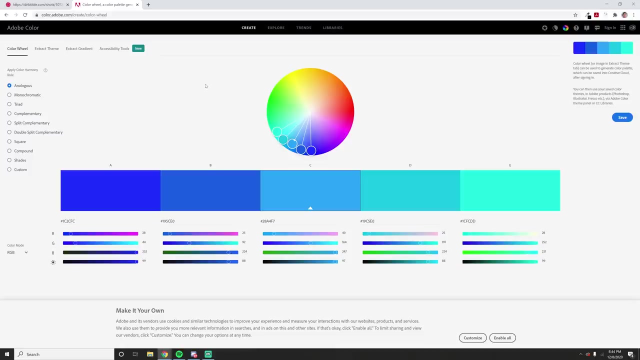 it should stop. a great resource to pick complimentary colors is adobe color, so search color adobe and here it is. first of all, we have inoculus, which basically represents you. pick a color like green and it's going to give you kind of the edges of that right, so kind of in that same range, and 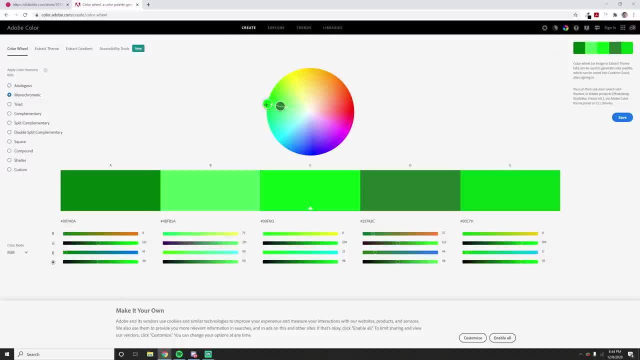 it's going to create you a color scheme. we have monochromatic, which we talked about. it's just going to give you a different shade of a color. that's going to give you kind of a differentering shade of a specific color that you pick. so here right, we have a a more desaturated version of this orange. 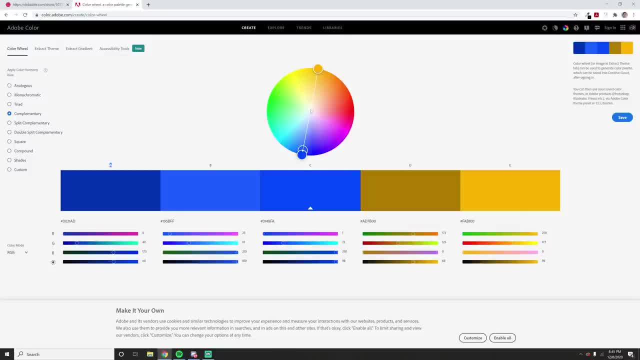 complementary is a very popular one, which basically means that you're going to pick a color and the other one is going to be on the other end of this hue spectrum here. all right, so if we go with blue, then we have orange. we're going to see this used in a bunch of movies as well. the mid 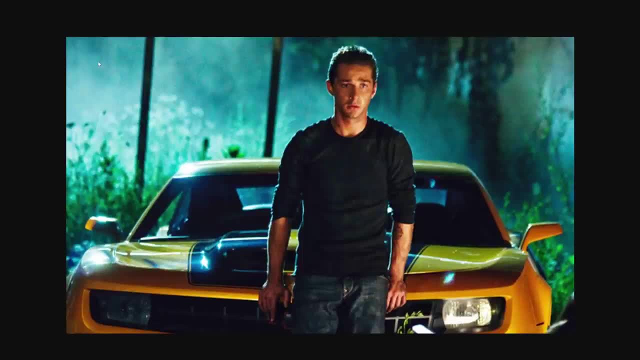 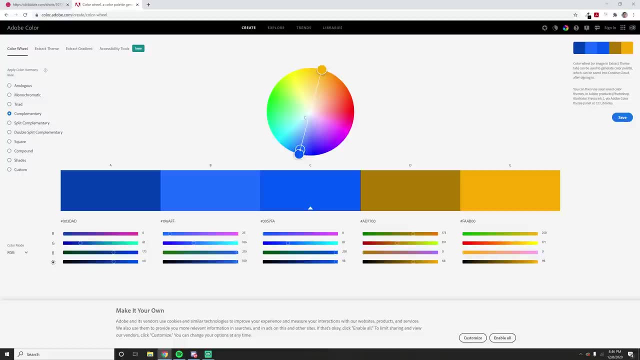 tones and the highlights are going to be orange, while the shadows are going to be bluish. and when you're using this complementary, you can pick one color as your primary, that you're going to be using a lot, and you can pick the orange as a secondary color, and there's a bunch of other ones.